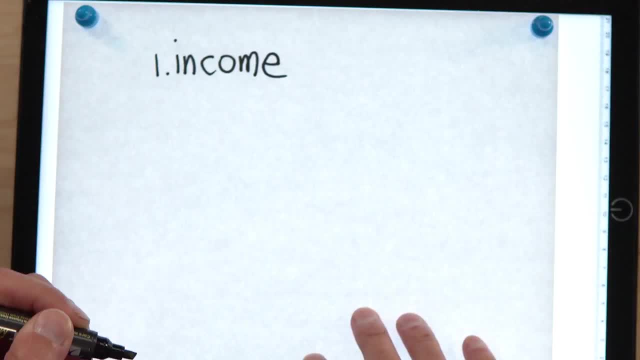 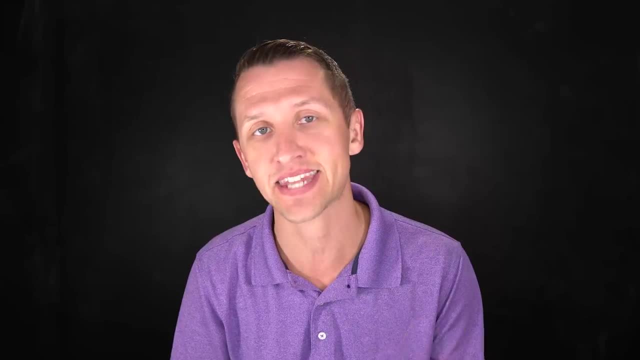 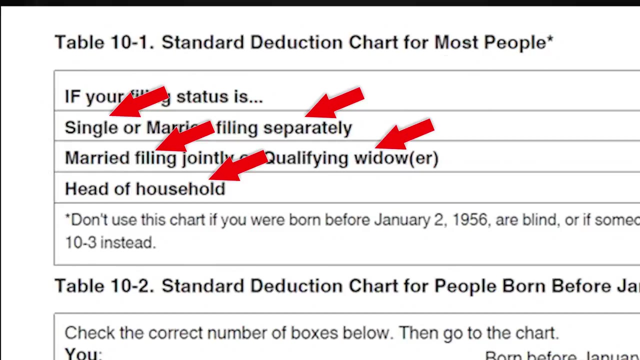 thousand dollars. Step two is figuring out your filing status Now. it could be single. married filing jointly, married filing separately, head of household, qualifying widow or widower. Now for this walkthrough: we're going to choose the filing status of single In step three now. 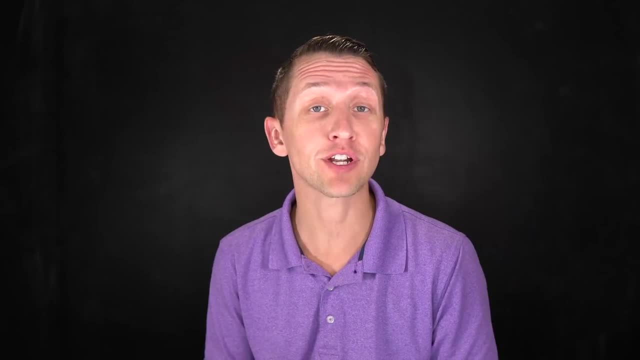 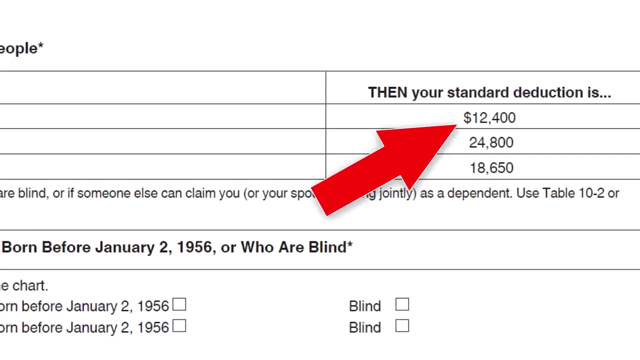 we need to figure out what our standard deduction is Now. we've already figured out our filing status. so for someone that's filing as single, it's 12,400. for the standard deduction For married filing jointly it would be $24,800 and for head of household it'd be $18,650.. So now we have $100,000. 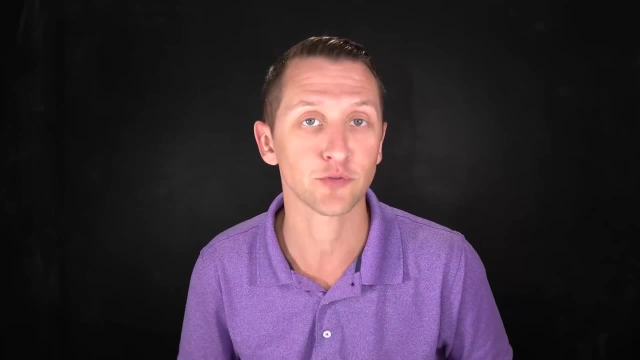 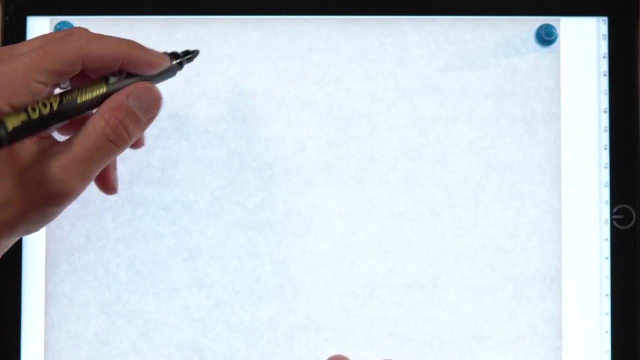 of income. We're filing a single and we have a standard deduction of $12,400.. So for step four, it's time to figure out our taxable income. So we're going to take our income of $100,000 and we're going to subtract our taxable income. So we're going to take our income of $100,000. 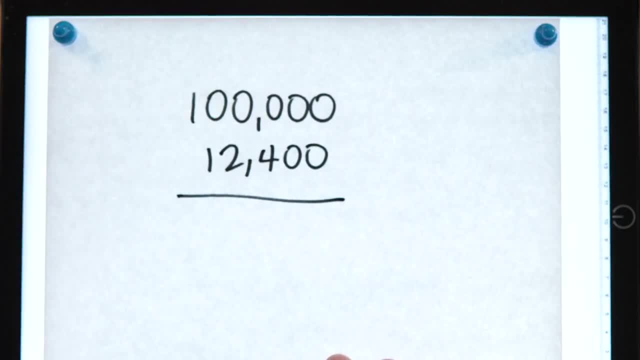 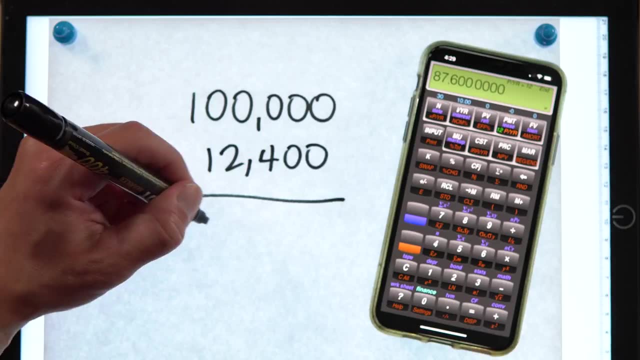 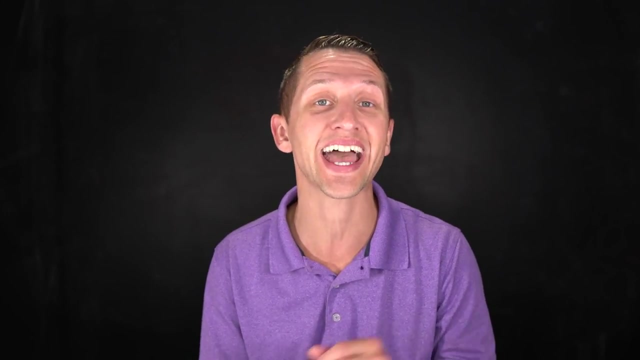 and we're going to subtract our standard deduction of $12,400.. So $100,000 minus $12,400 gives us a taxable income of $87,600.. And now it's time for step five, to figure out our tax liability, or to estimate our taxes. Now we're going to use publication 17.. Now, if you haven't, 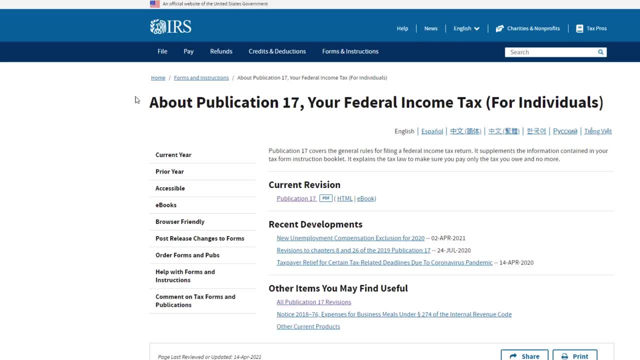 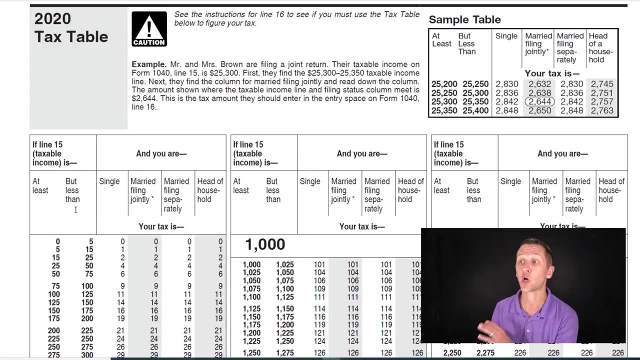 ever heard of publication 17,. it's the IRS's guide to your individual taxes, And at the end of this video there's a quick cheat sheet to figure out your tax liability. Now we already have all the information that we're going to need, So what we can see here is we can see that it's broken down. 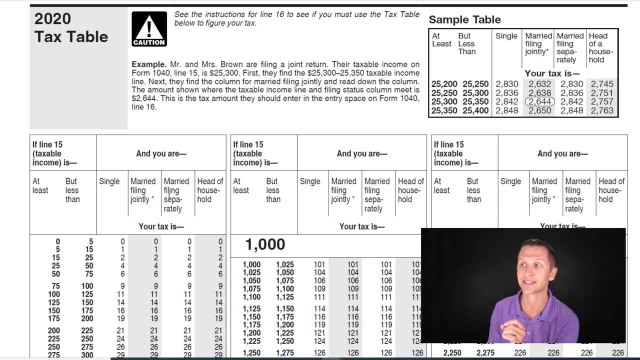 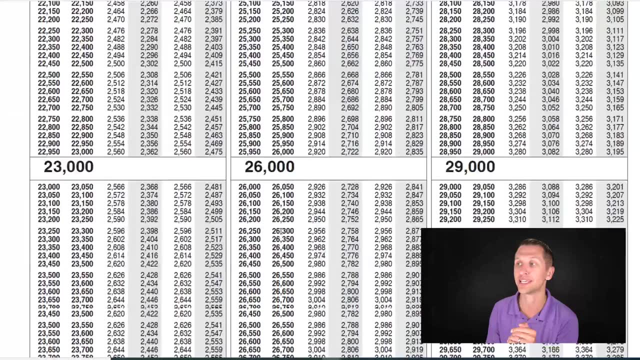 on your filing status- If you're single, married, filing jointly, separately or head of household- and what your taxable income is. Not your income, but the calculation that we just went through, which is subtracting your standard deduction. So if we scroll down we can go to the $87,600.. 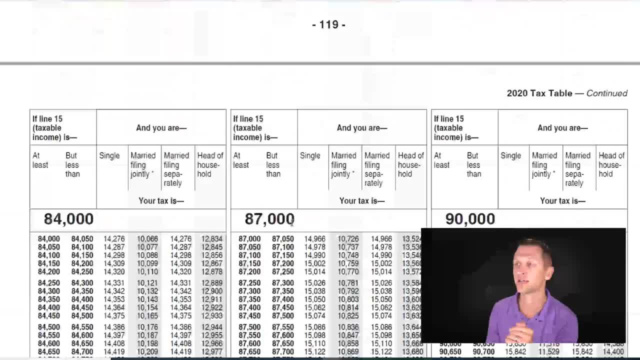 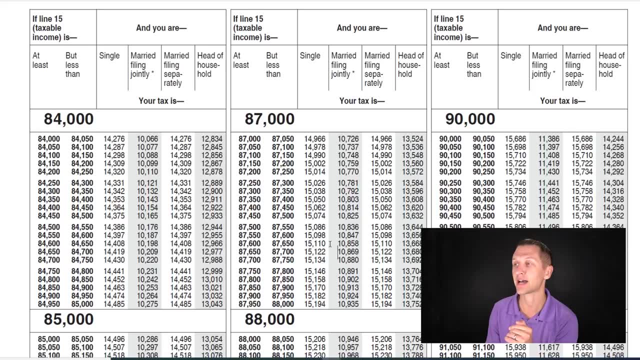 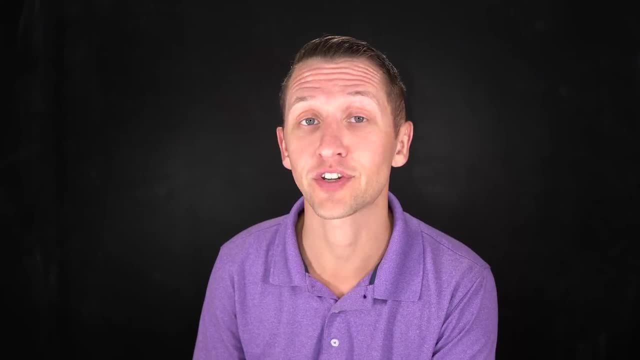 Scroll all the way down and we will see. $87,600 has a total tax liability right there of $15,110 for someone that's filing as single. If your income is over a hundred thousand dollars, there's another cheat sheet right here that we can scroll down to and we can go through that. 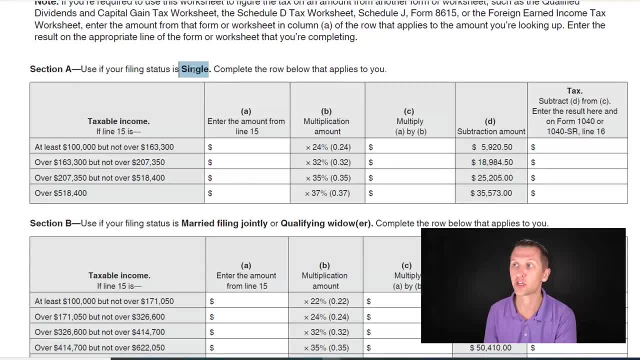 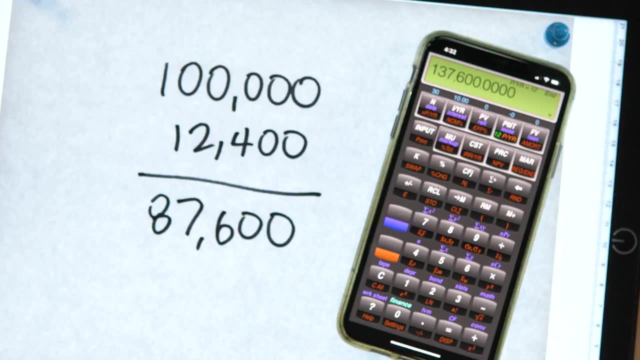 So this is based on your filing status as well. So if we see up here, it says single, So let's change our tax liability to $150,000, which is over a hundred thousand dollars of taxable income. So if we take our $150,000 now and we subtract our $12,400, that's going to give us a taxable. 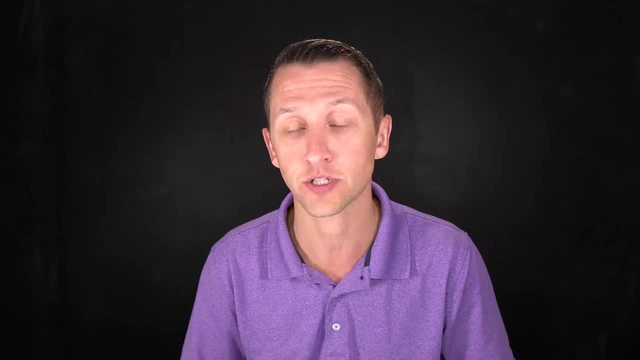 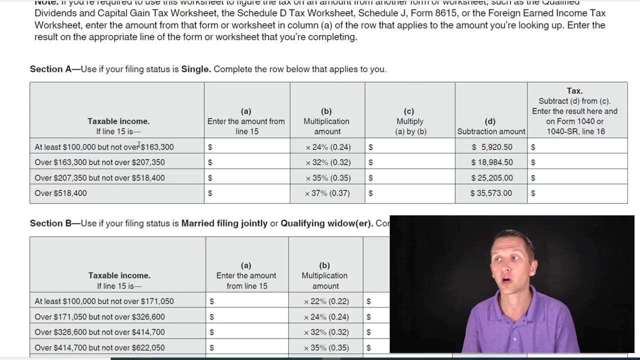 income of $137,600.. So if we go to this chart right here, we could see that that first line at least a hundred thousand, but not over $163,300.. That means we can use this first line. So we want to. 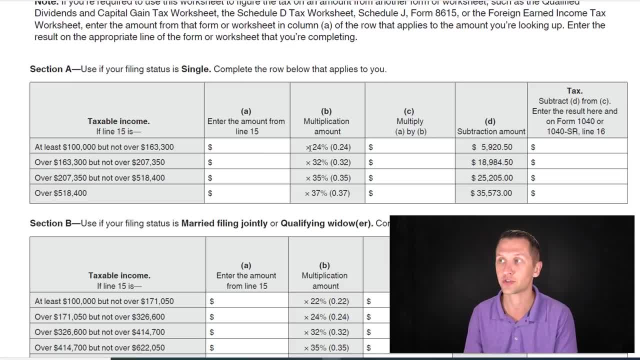 multiply our $137,600 by 0.24 or 24%, So we can multiply it by 0.24, and that's going to give us $33,024.. And, moving over to the next column, all we need to do is subtract that amount. 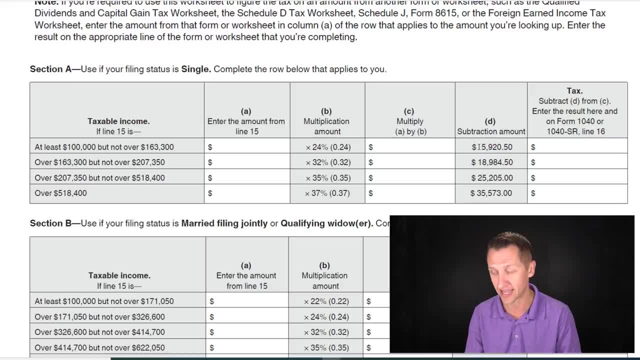 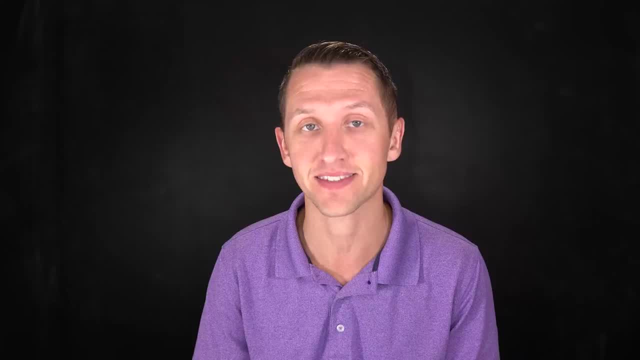 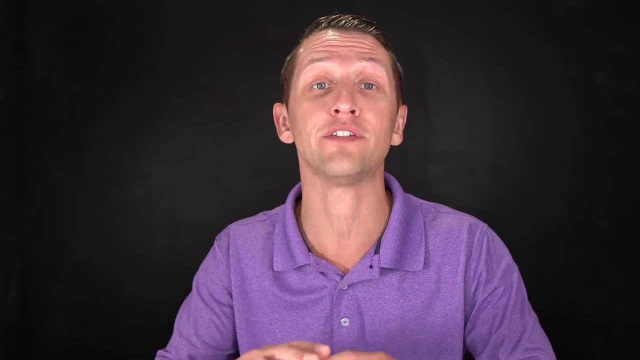 which is $5,920.50, giving us a total tax liability estimate of $27,103.50.. Now the reason that I'm calling this an estimate, because it doesn't account for long-term capital gains, qualifying dividends or any of your credits or other deductions that you might qualify for. But this is a quick way.